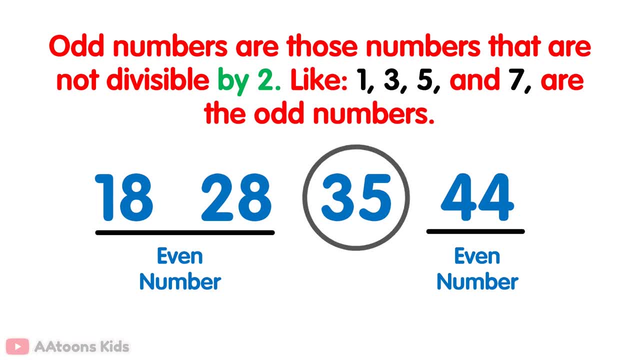 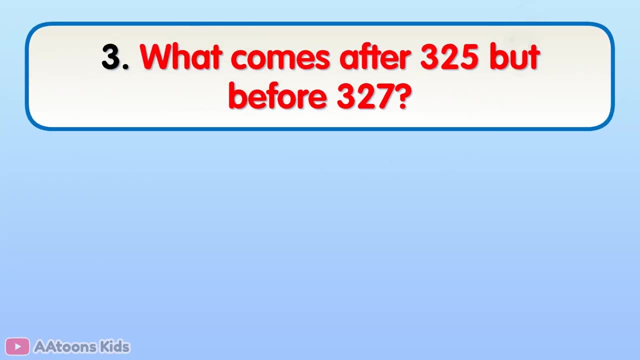 Except 35, all the numbers are even numbers That are exactly divisible by 2.. So 35 is an odd number. For more concepts on even and odd numbers, watch the video link in description. What comes after 325 but before 327?. 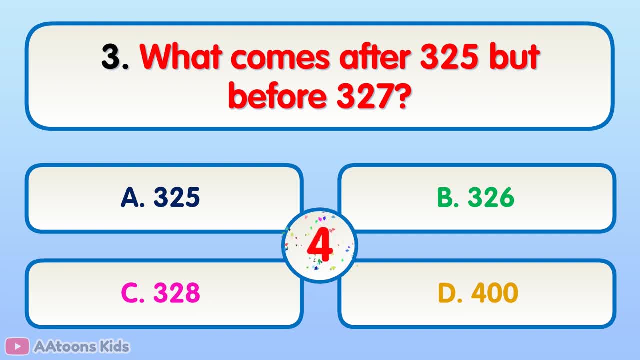 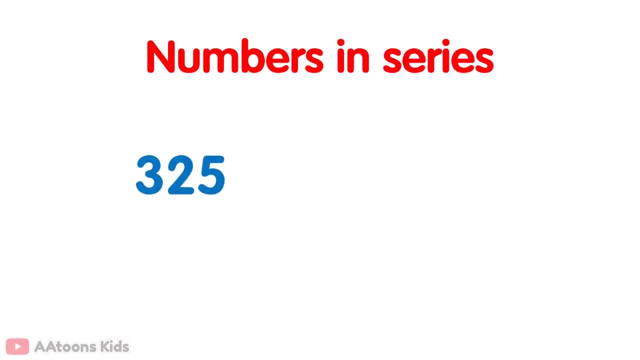 326 When we count the numbers in series 325-326-327.. 326 comes between 325 and 327.. 326 comes in the series 325-426-N3.. 326 comes between 325-0275.. 326 comes between 2.. 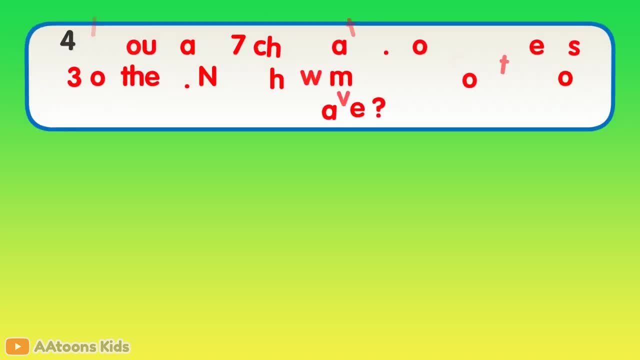 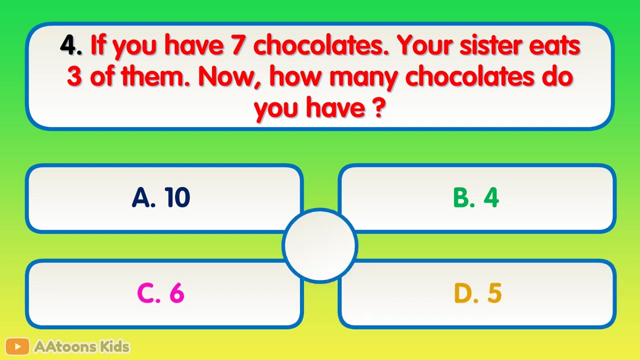 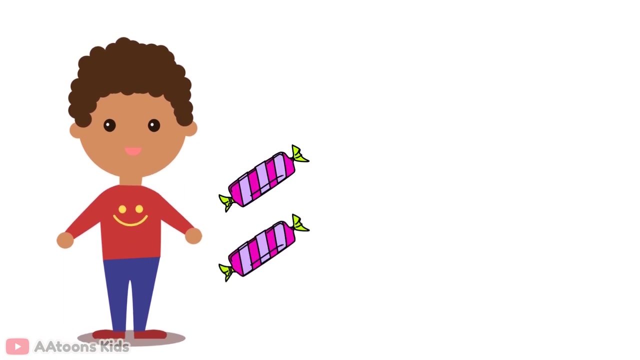 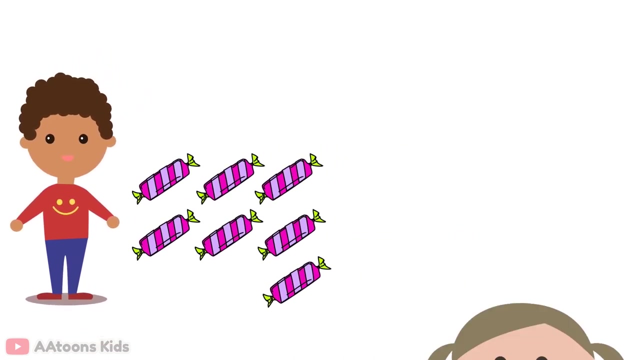 327 comes after 1.. 1. 1. If you have 7 chocolates, your sister eats 3 of them. Now, how many chocolates do you have 4 chocolates. You have 7 chocolates. Your sister eats 3 of them. 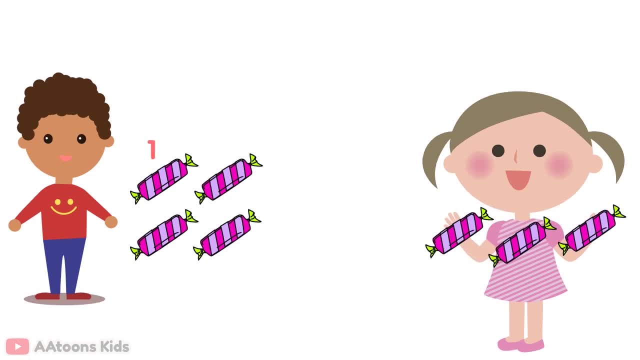 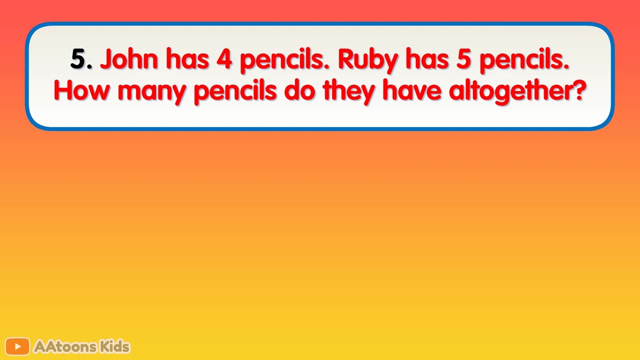 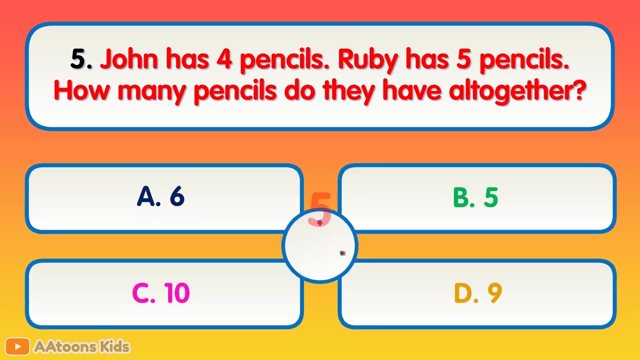 Now let's count how many you have left: 1,, 2,, 3,, 4. You have 4 chocolates left. John has 4 pencils, Ruby has 5 pencils. How many pencils do they have altogether? 9. 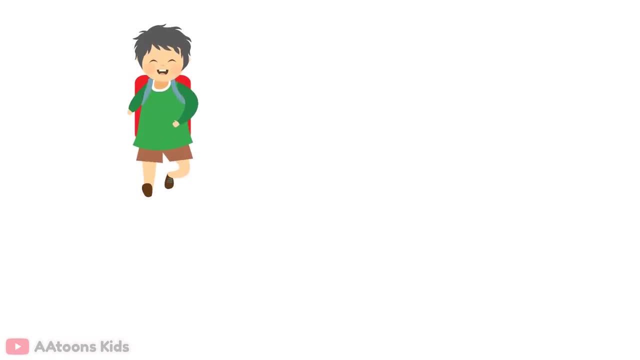 John has 4 pencils: 1,, 2,, 3,, 4. Ruby has 5 pencils: 1,, 2,, 3,, 4, 9, 5. Let's count together: 1,, 2,, 3,, 4,, 5,, 6,, 7,, 8,, 9. 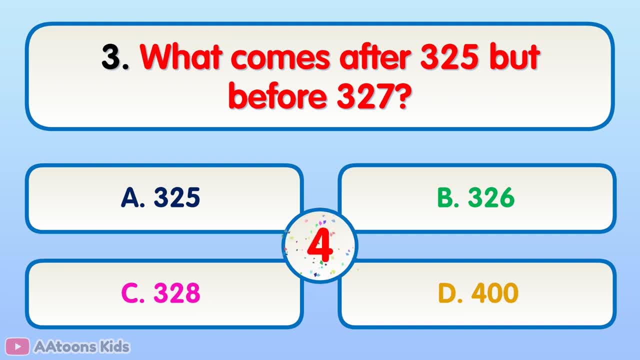 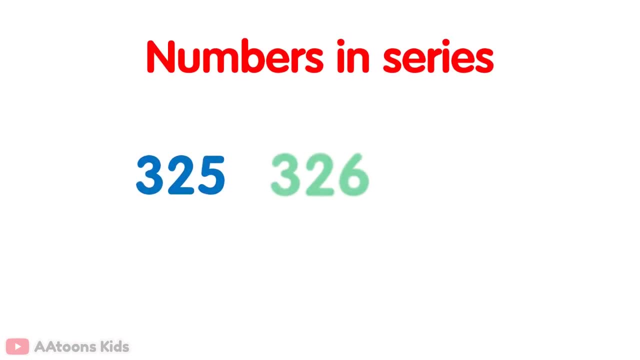 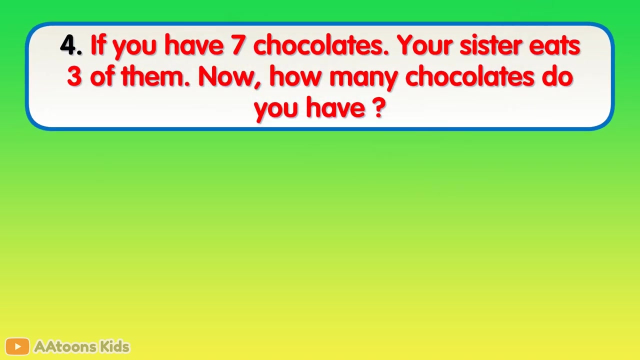 326.. When we count the numbers in series, 325, 326, 327.. 326 comes between 325 and 327.. 327. If you have 7 chocolates, your sister eats 3 of them. Now, how many chocolates do you have? 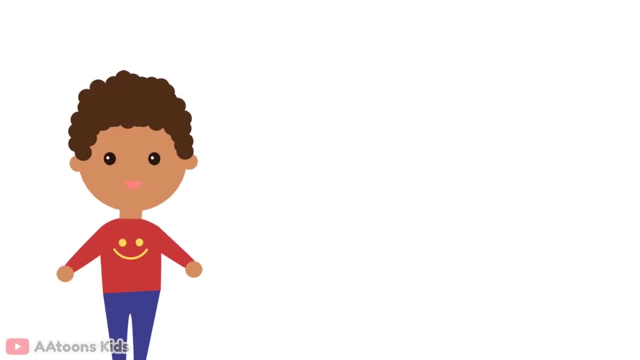 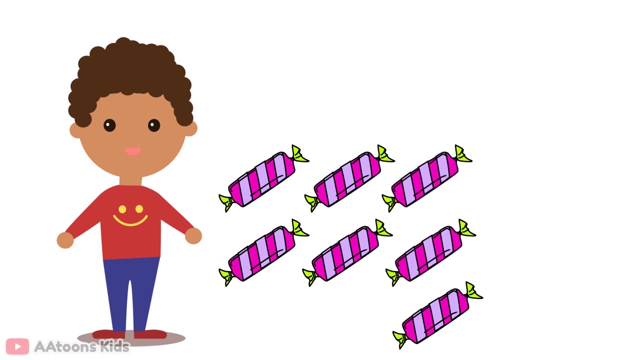 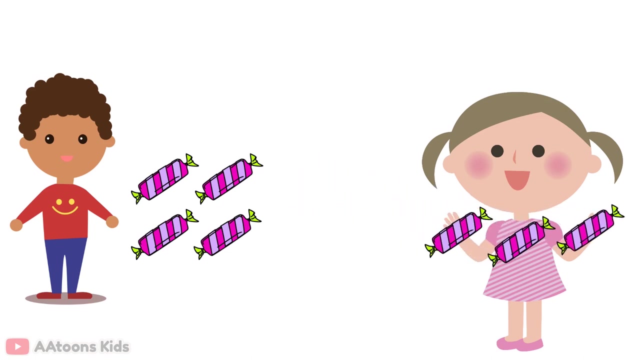 4 chocolates. You have 7 chocolates. Your sister eats 3 of them. Now let's count how many you have left: 1,, 2,, 3,, 4. You have 4 chocolates left. John has 4 pencils. 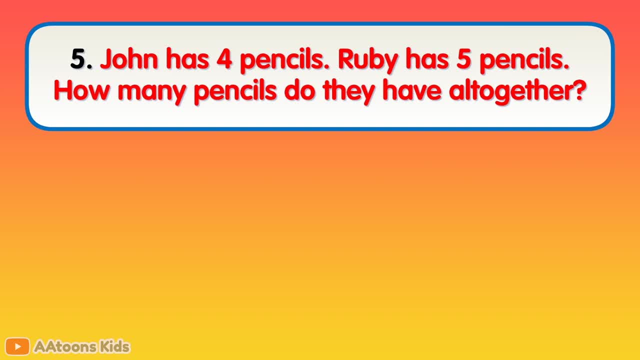 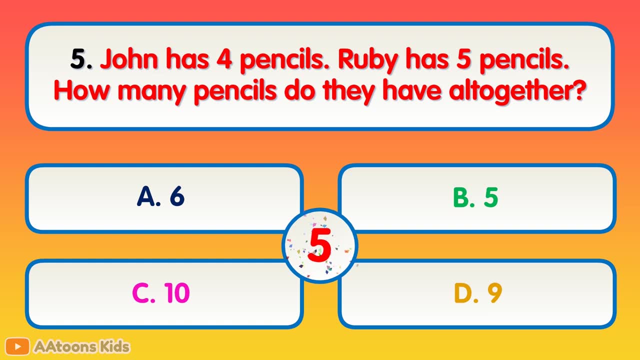 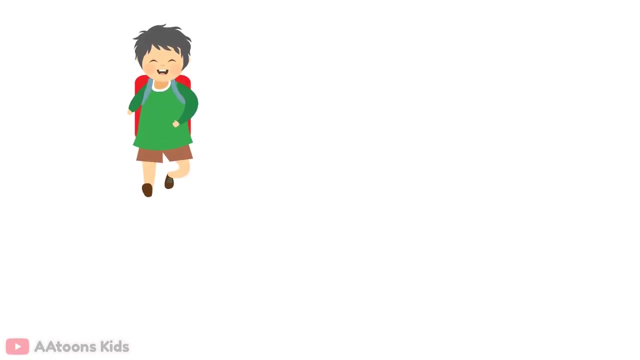 Ruby has 5 pencils. How many pencils do they have altogether? 9. John has 4 pencils: 1,, 2,, 3, 4. Ruby has 5 pencils: 1,, 2,, 3,, 4, 9. 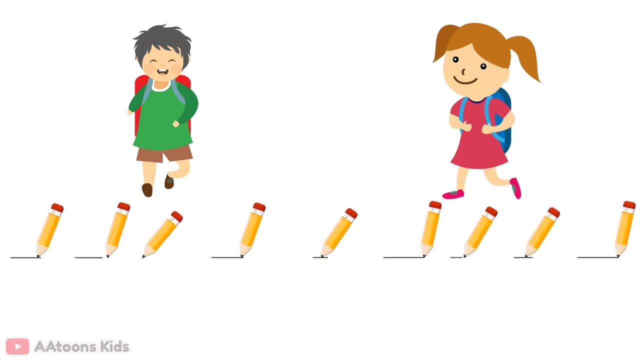 5. Let's count together 1,, 2,, 3,, 4,, 5,, 6,, 7,, 8,, 9. All together they have 9 pencils. Ram bought 2 dozens banana for Rs 20. 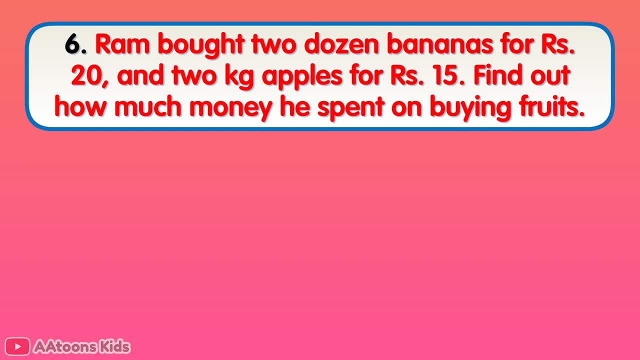 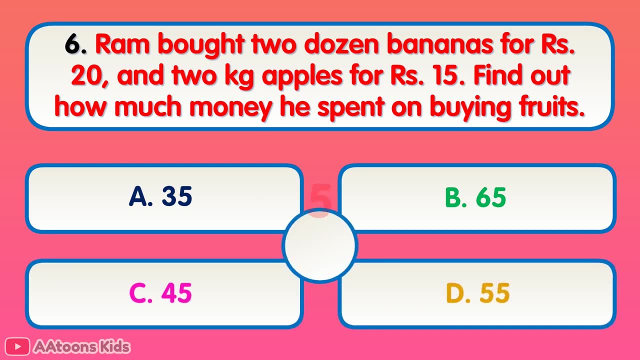 and 2 kg apples for Rs 15.. Find out how much money he spent on buying fruits. You should steal all fruits before you buy some Home production costs. family stock 35. you can't find the fruits available on E-book Variant: Gosh darn. 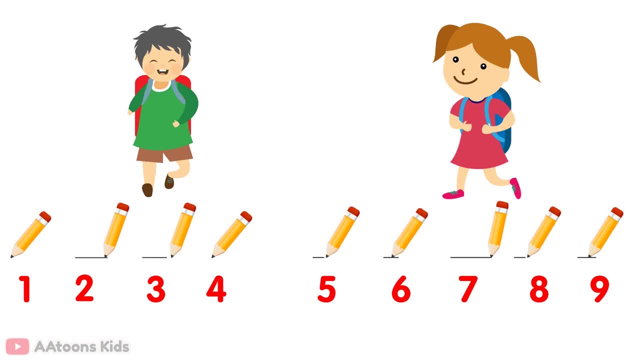 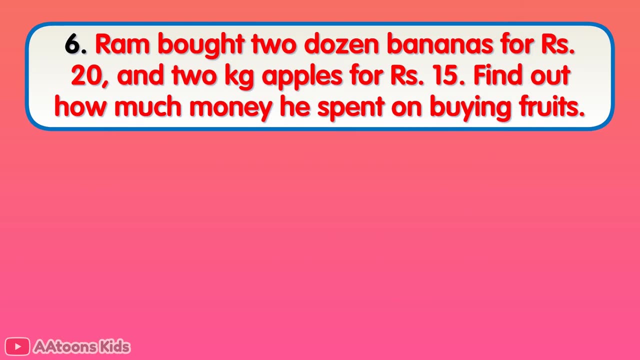 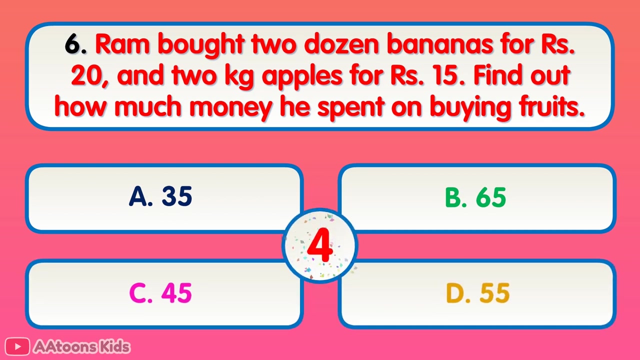 All together, they have 9 pencils. Ram bought 2 dozens banana for Rs 20 and 2 kg apples for Rs 15.. Find out how much money he spent on buying fruits. If you are using my application, you will like it. 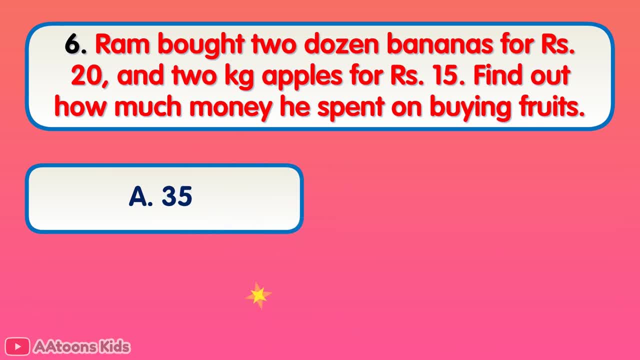 You are also allowed to Mortgage for fruits. This is also face-to-face, But in this video we have берき to home- courts. Put 3 oceans of bananas on four sleeves. Everyika will also be depicted with the price. 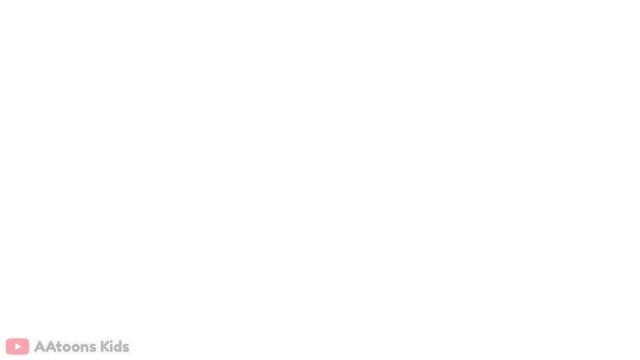 I have prepared it. On which fruits do they get the total amount You would get one sweet costs 5 crore. You have to earn 1 crore from your payment 3. They will be for 2 and 2. During the question of where the fruit comes from or after their Target of causing soy-cups. we have three. fica combine 23 am. 2 haba double potato costs 36. itself is equal to 5 percent. 2 B playgrounds could be mooi, But we know each banana has a stuffed fruit type. 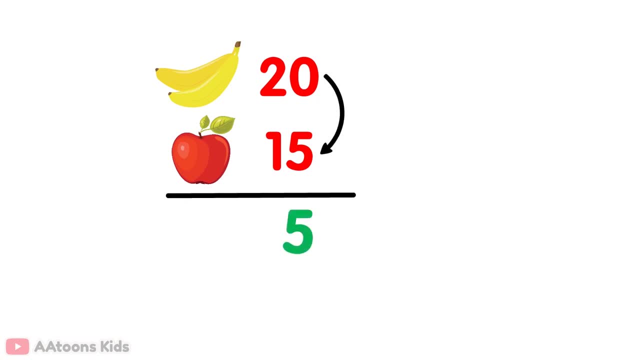 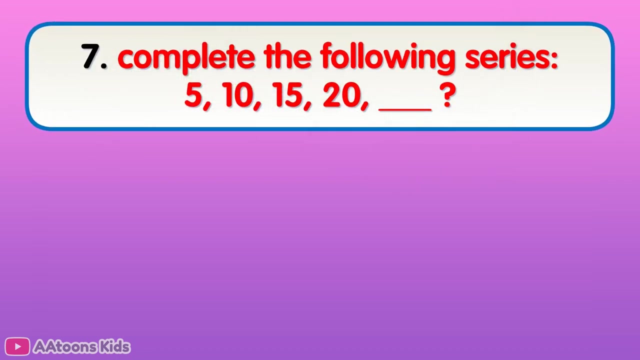 Now add: 0 and 5 are 5, 2 and 1 are 3, 35. Ram spends 35 rupees on buying fruits. Complete the following series: 5,, 10,, 15,, 20.. 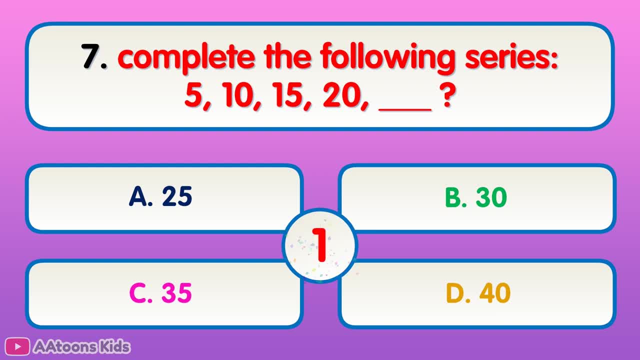 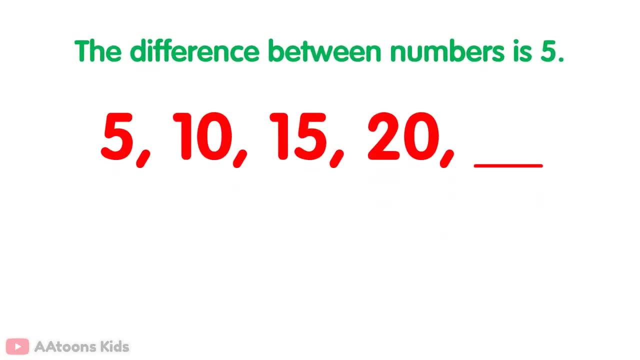 25,. the difference between numbers is 5,. 5 is added in 5, it becomes 10,. 5 is added in 10, it becomes 15,. 5 is added in 15, it becomes 20.. In the same way, again, 5 is added in 20, it becomes 25.. 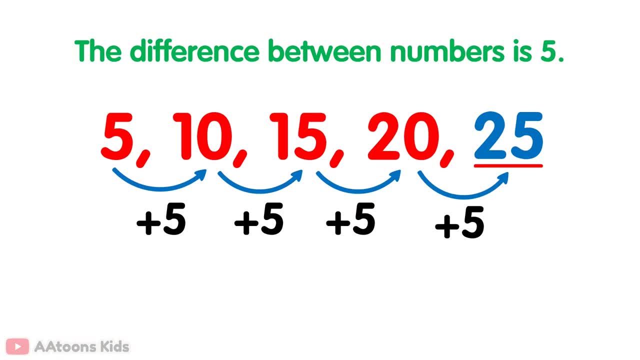 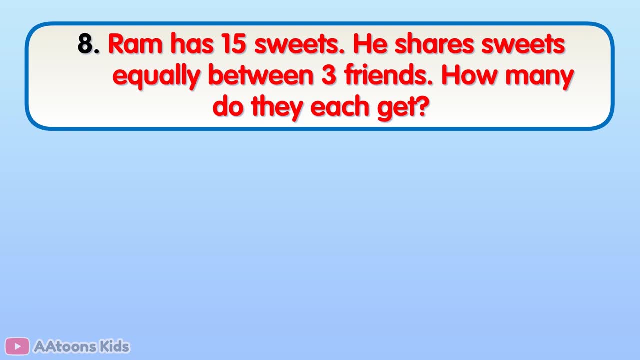 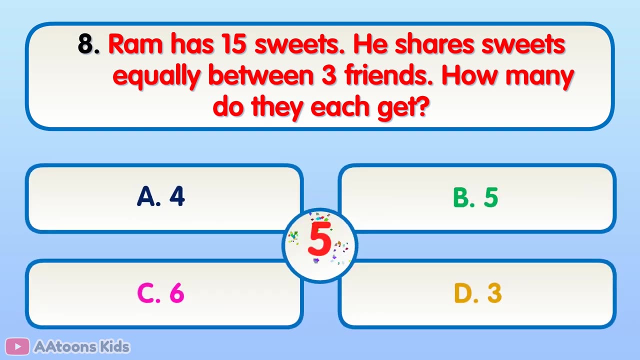 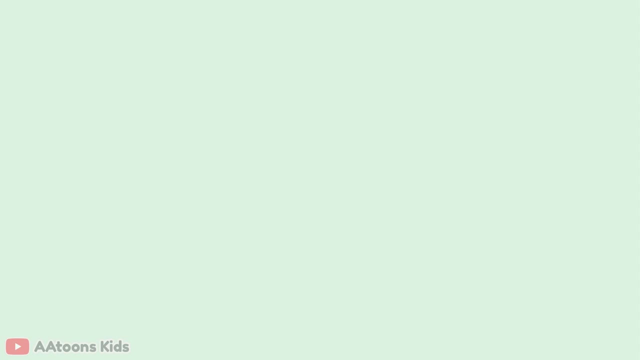 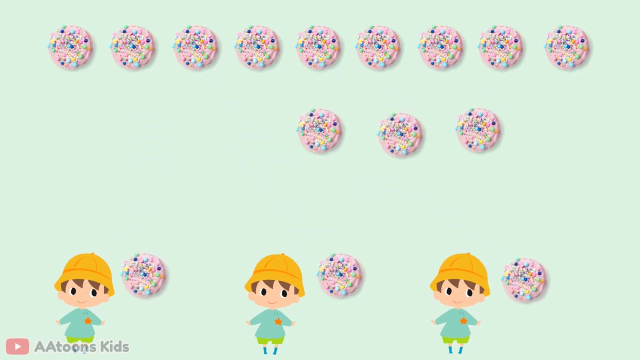 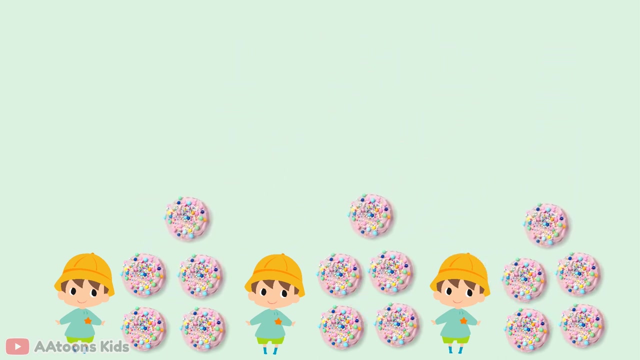 So the answer is: Ram has 15 sweets. He shares sweets equally between 3 friends. How many do they each get? 5. Sharing sweets: Sharing means dividing. Divide the 15 sweets between 3 friends. Each friend gets 1,, 2,, 3,, 4,, 5 sweets. 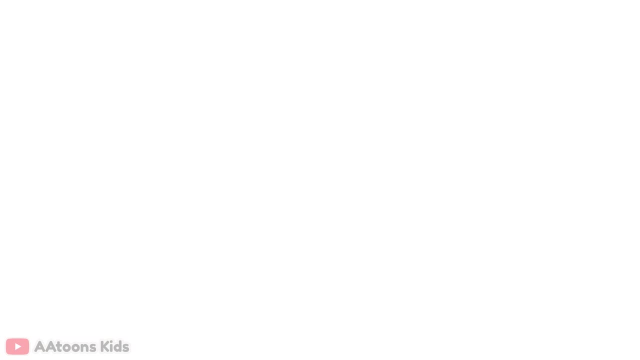 2 fruity cr сделать fruit. We have to add the cost of all fruits to get the total amount. For u don't buy all of these scare. 1 hundred mos 전에, 2 dozen bananas is equal to 20 rupees. 2 kg apples is equal to 15 rupees. 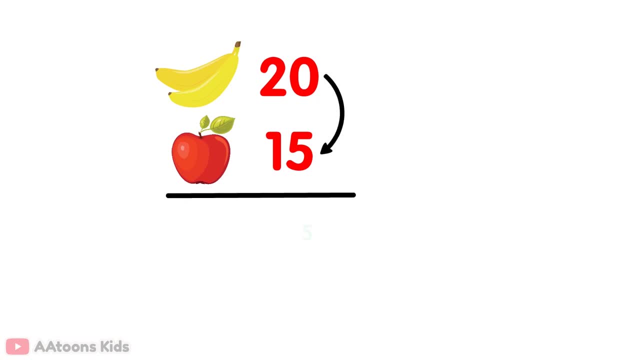 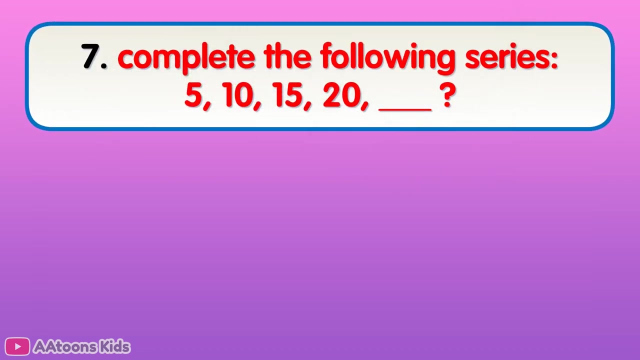 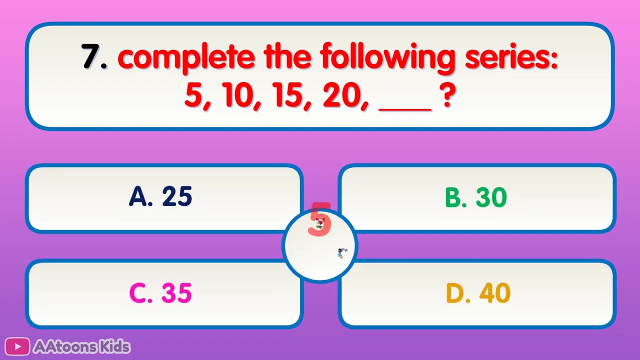 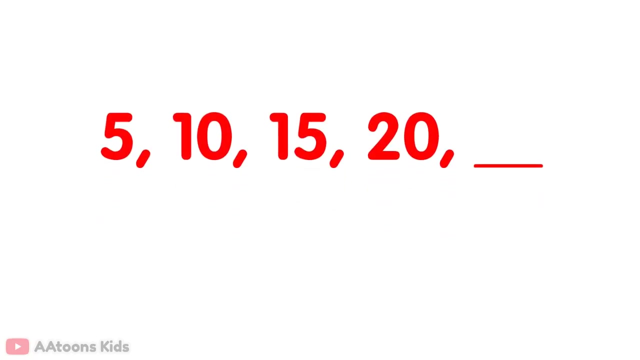 That's 50 tons of fruits. now add 0 and 5 are 5, 2 and 1 are 3. 35 ram spends 35 rupees on buying fruits. complete the following series: 5, 10, 15, 20, 25. the difference between numbers is 5. 5 is added in 5, it becomes 10. 5 is added in 10, it becomes 15. 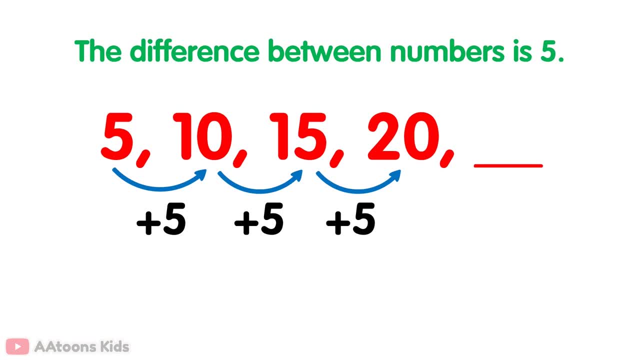 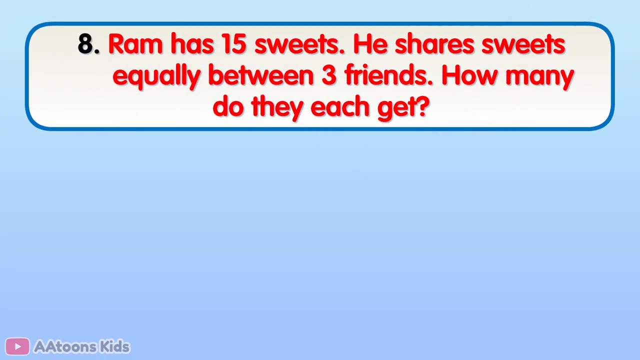 5 is added in 15, it becomes 20. in the same way, again 5 is added in 20, it becomes 25. so the answer: 25.. ram has 15 sweets. he shares sweets equally between three friends. how many do they each get? 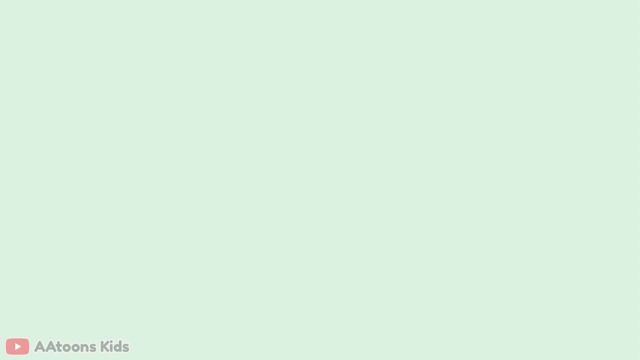 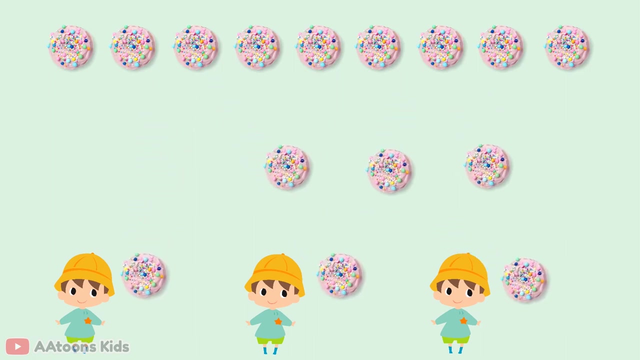 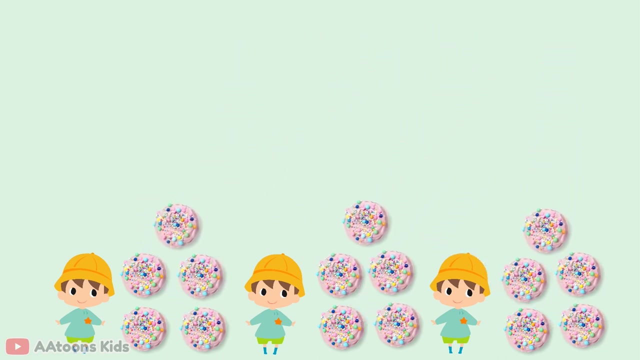 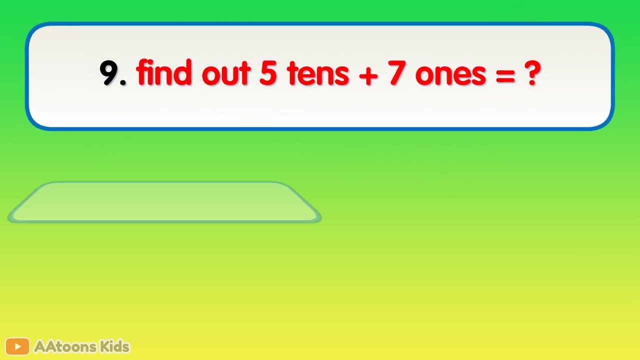 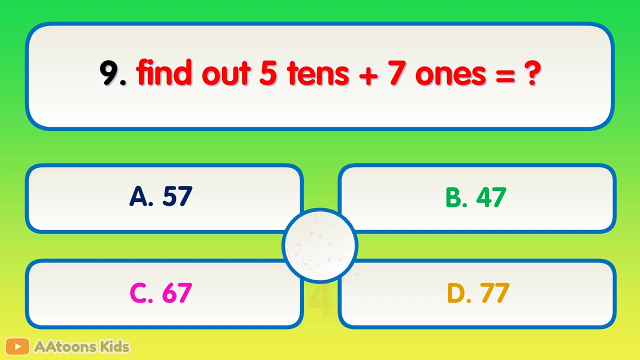 five. sharing with dividing. divide the 15 suits between three friends. each friend gets one, two, three, four, five, six. you have to divide 15 by three. you will get five. find out five. tens. seven ones. find out five. 10s means five multiplied by 10. so five 10s are 50.. 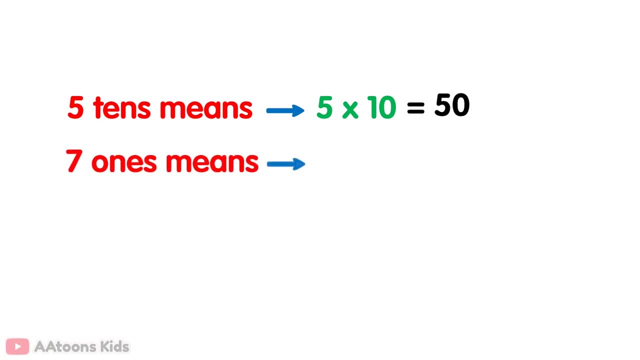 seven. means 7 multiplied by 1 is 7. now add 50 and 7. addition of 50 and 7 is 57.. now add 50 and 7. addition of 50 and 7 is 57.. now add 50 and 7. addition of 50 and 7 is 57.. 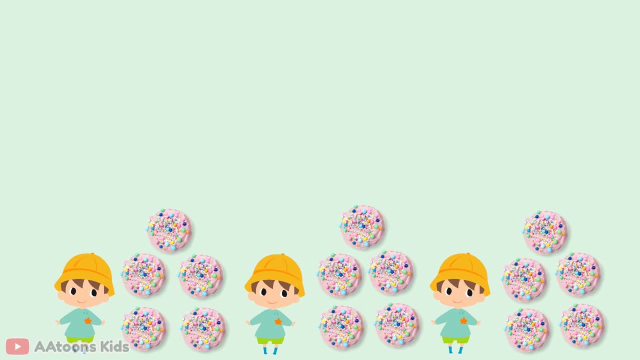 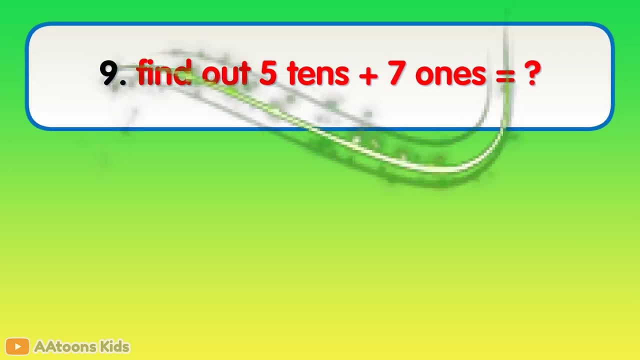 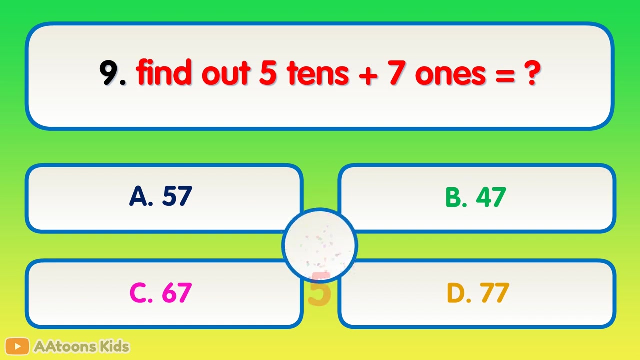 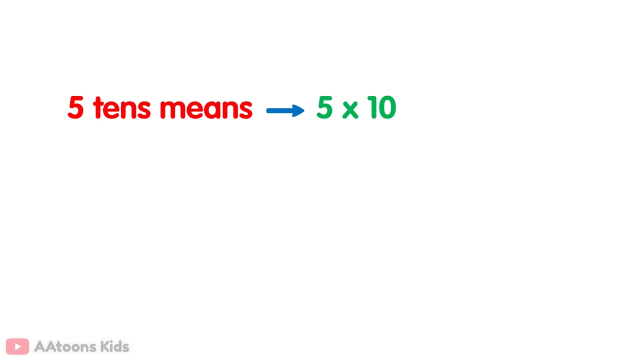 You have to divide 15 by 3. You will get 5.. Find out 5, 10s, 7, 1s For you, 50, 1s, Outro 57.. 5: 10s means five multiplied by 10.. 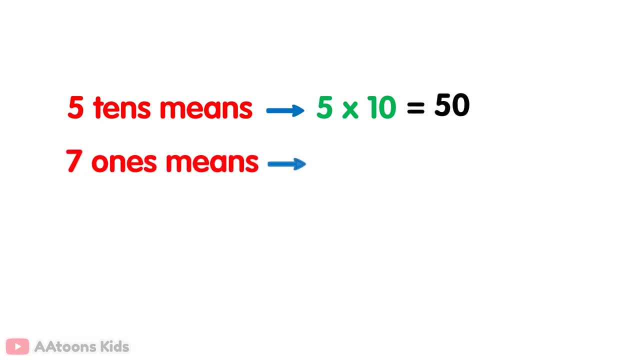 So 5- 10s are 50.. 7- 1s means 7 multiplied by 1 is 7.. Now add 50 and 7.. Addition of 50 and 7 is 57.. Addition of 50 and 7 is 57.. 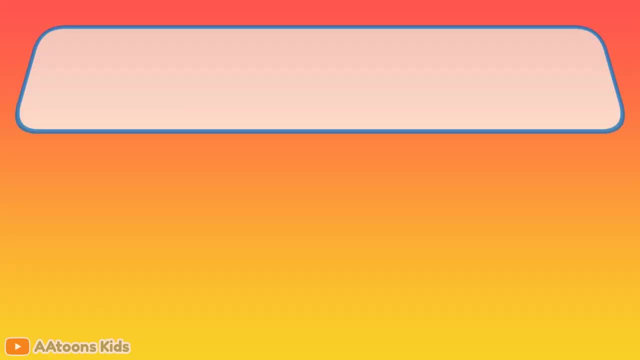 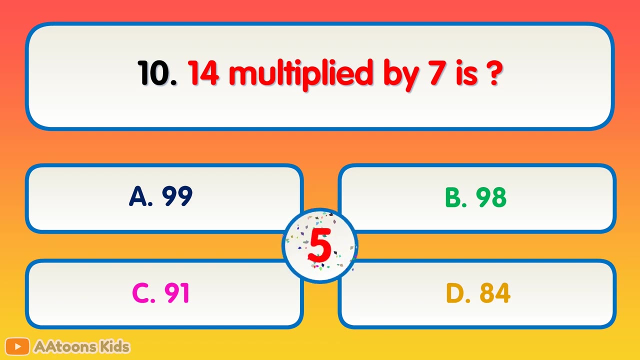 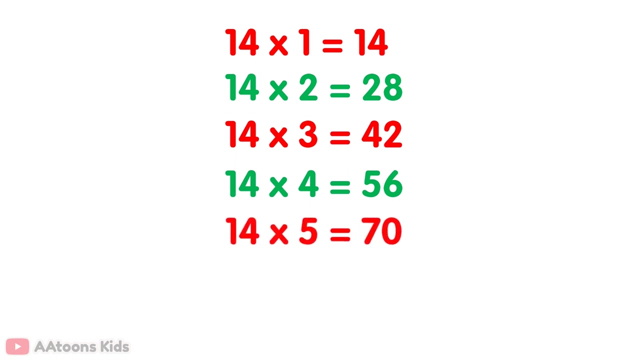 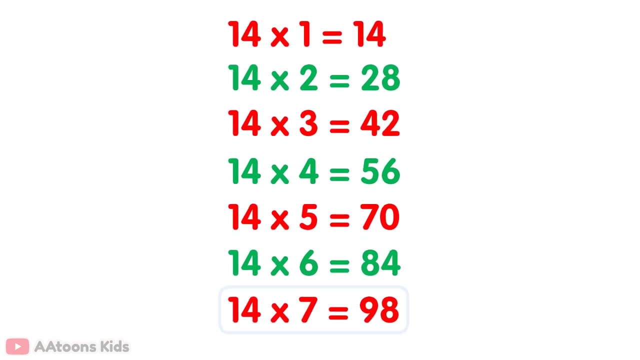 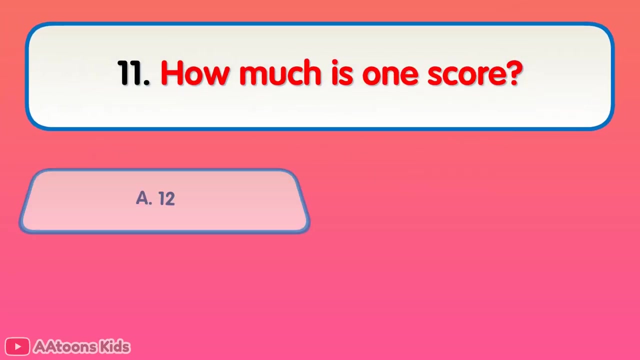 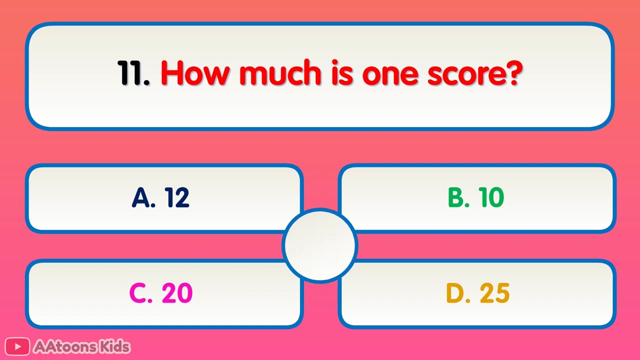 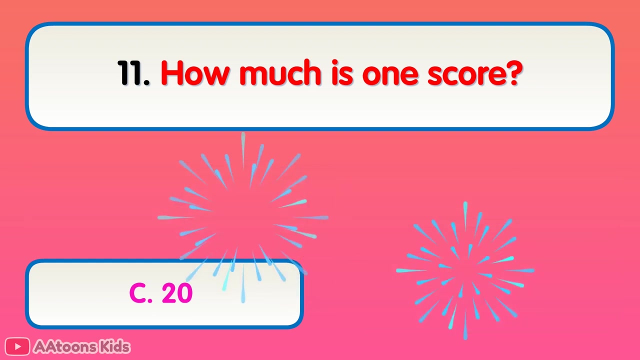 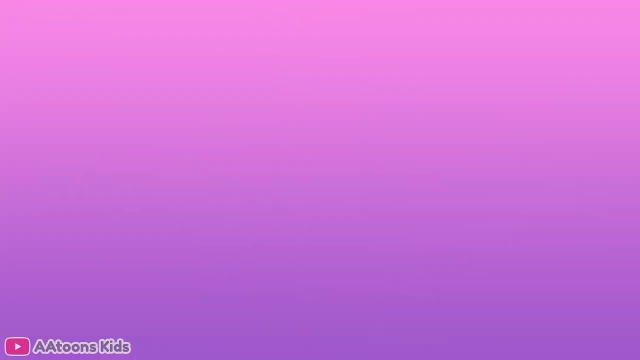 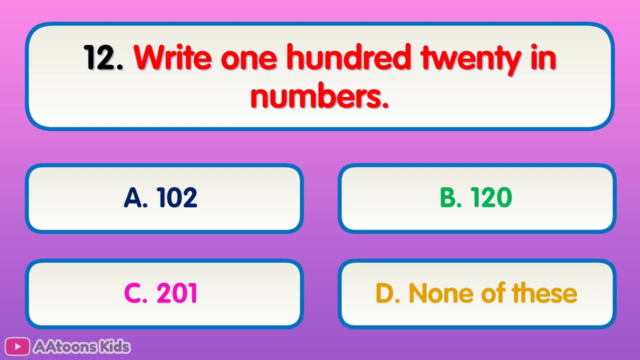 14 multiplied by 7 is 98. Let's count the table: 14 multiplied by 7 is 98. How much is one score? 14 multiplied by 7 is 98: 20. One score is 20. Write 120 in numbers. 20 multiplied by 7 is 98. 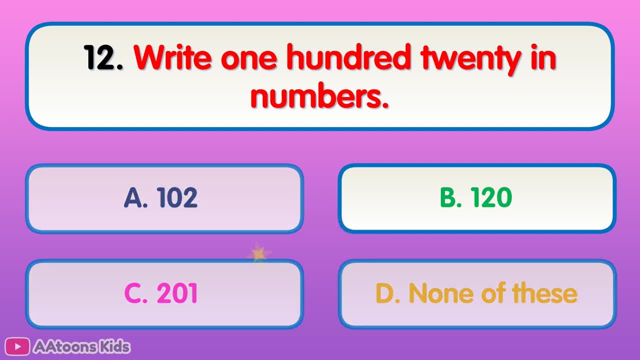 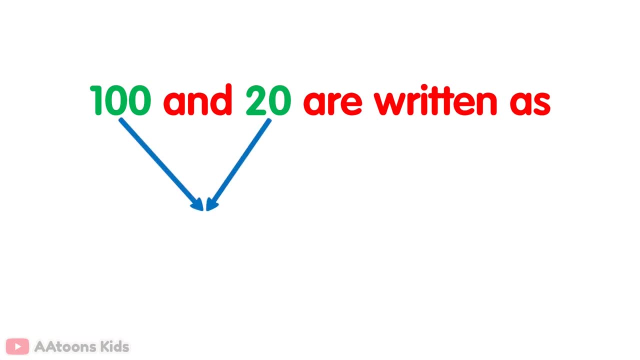 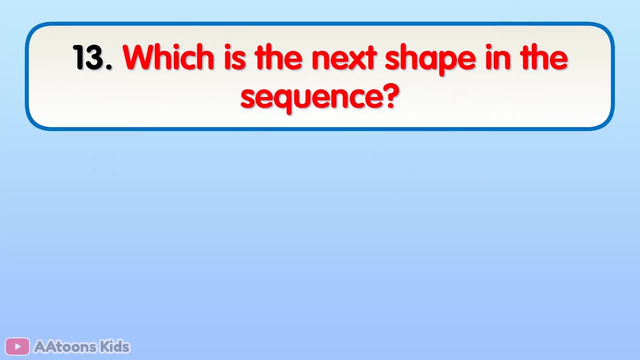 How much is one score? 20 multiplied by 7 is 98. How much is one score 120? 120 are written as 120. 120 are written as 120, Which is the next shape in the sequence. which is the next shape in the sequence? 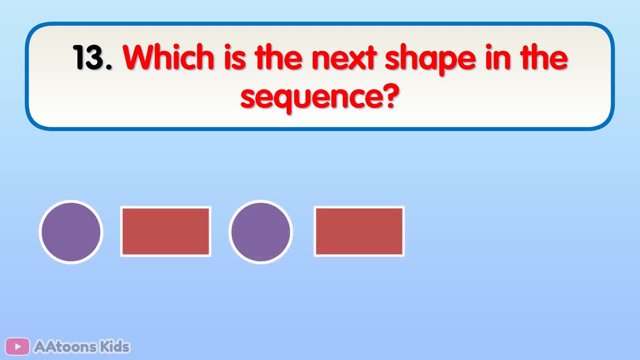 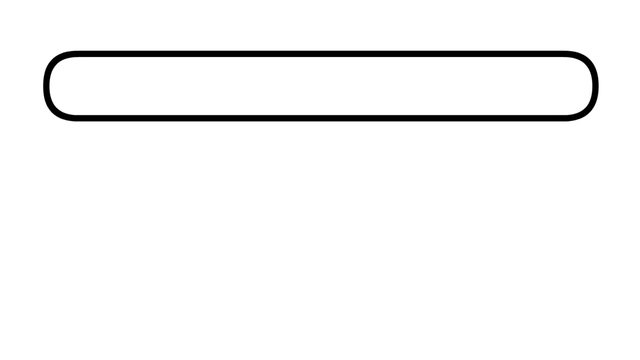 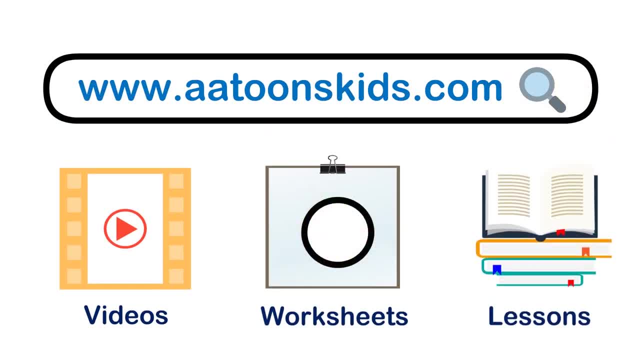 the 8th forts is Ki. the length of therest part will be Pot. 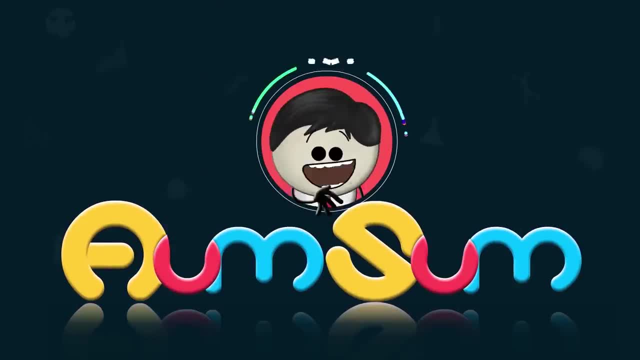 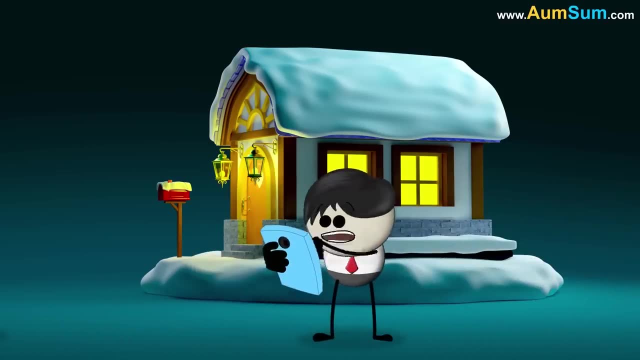 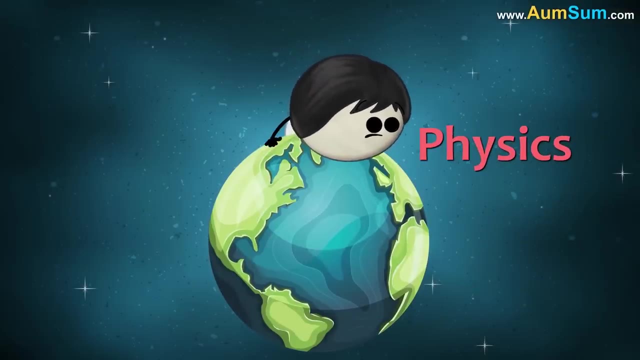 It's AumSum Time. What if there was no gravity on earth? No Problemo, I will order my burger from space. Oh, AumSum. From purely physics point of view, there would be no earth left, as no gravity means no mass. 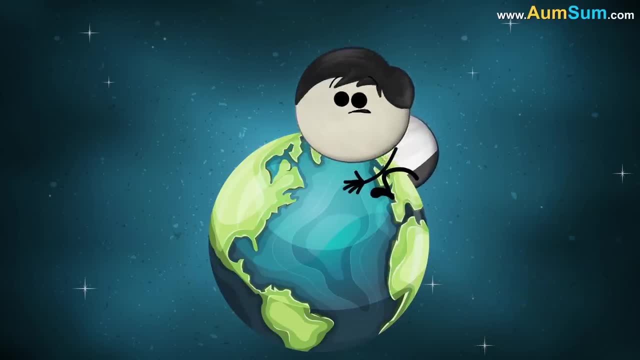 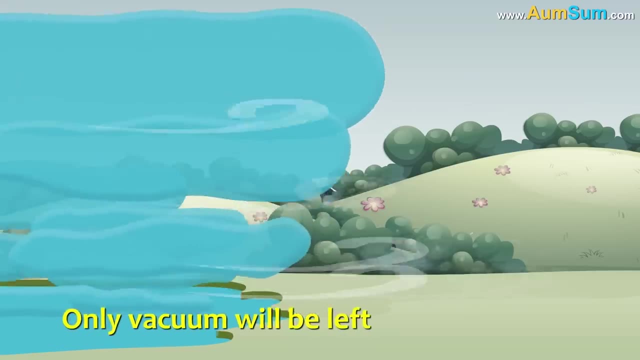 But leaving this point aside, let's see what else will happen. Oceans, rivers and lakes will float away, Entire atmosphere will vanish. only vacuum will be left. Everything on the surface of the earth, including humans, cars, rocks, etc. 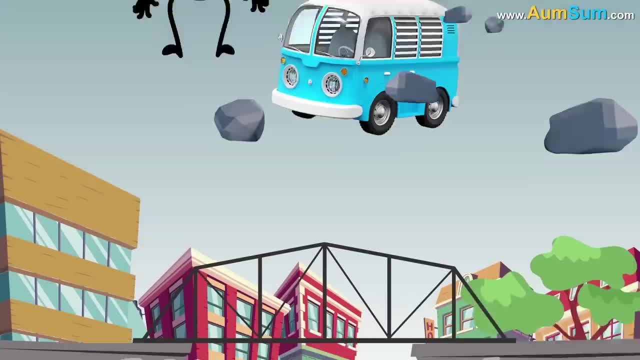 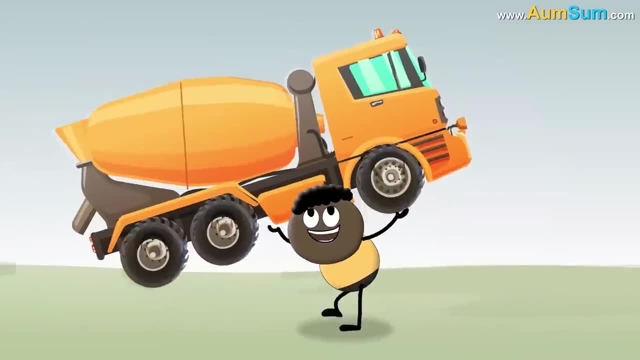 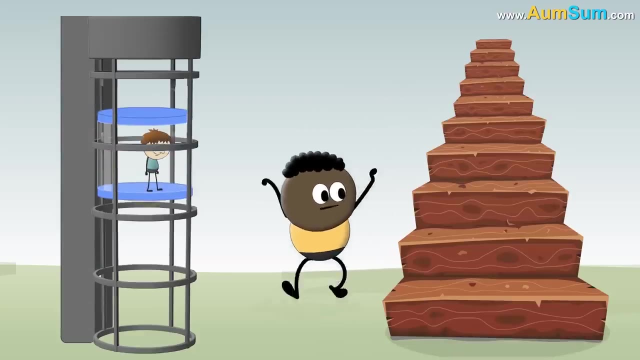 Will become weightless and float away into space. Things that are rooted into earth, like trees, bridges and buildings, will remain, But not for long. On a funnier note, anybody will be able to lift heavy weights. Football will become a one-kick game and there will be no need of stairs or elevators. 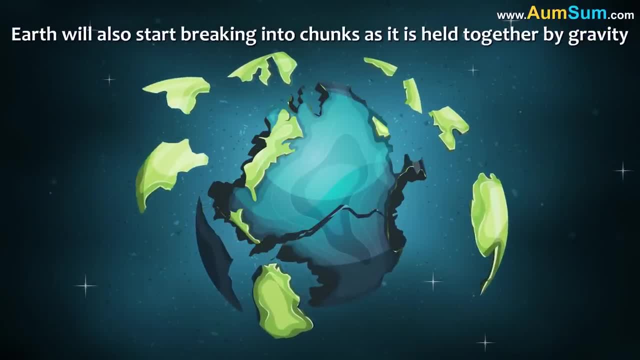 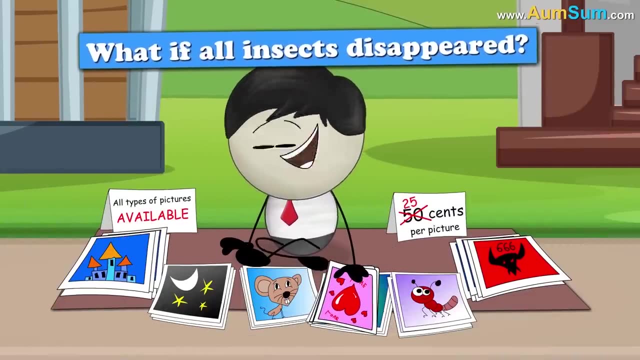 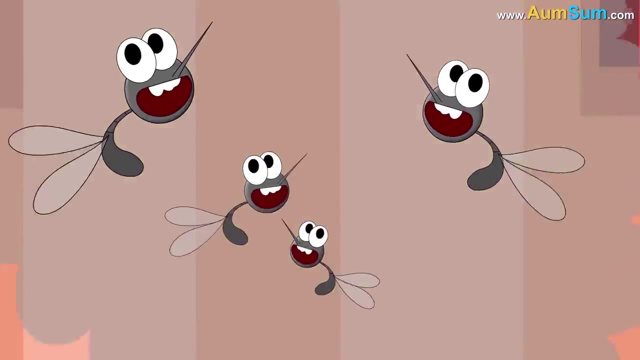 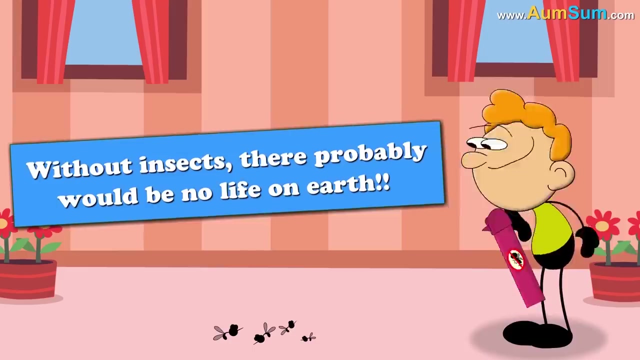 Finally, earth will also start breaking into chunks, as it is held together by gravity. What if all insects disappeared? No worries, I have their photographs. You might think insects are inconsequential, But the reality is. without them, there probably would be no life on earth. 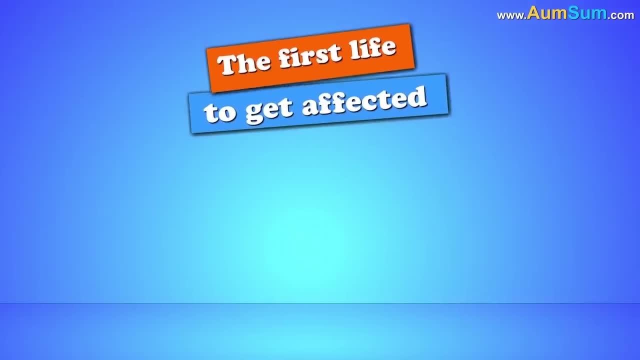 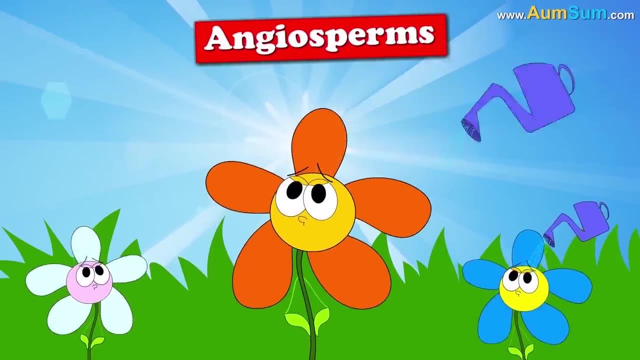 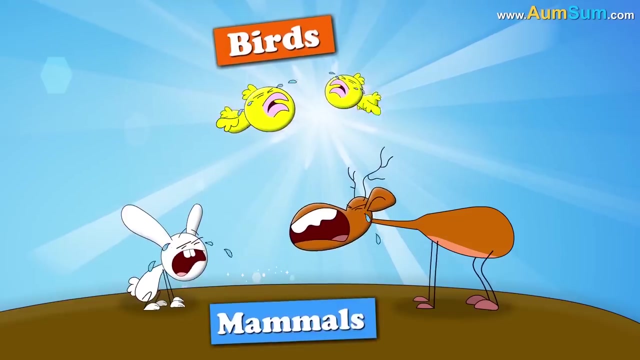 The first life to get affected would be plant life. Most plants in the world are angiosperms, that is, flowering plants. Without insects pollinating them, plant life would gradually disappear. Gradually, birds and mammals feeding on plants would also disappear.